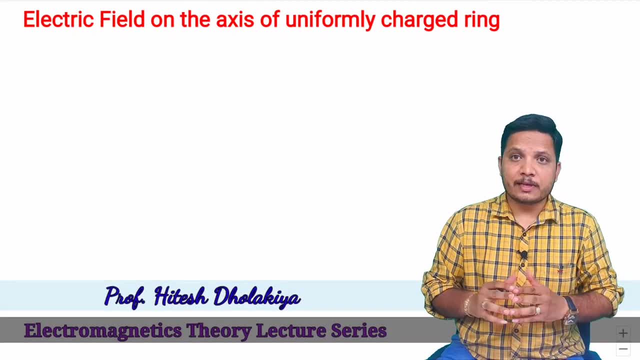 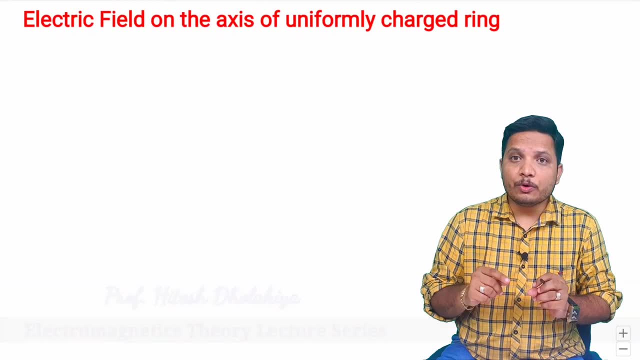 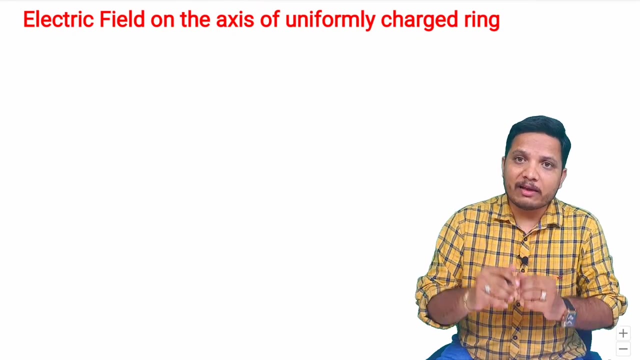 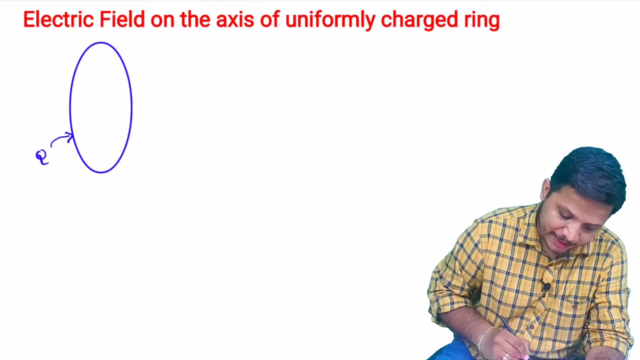 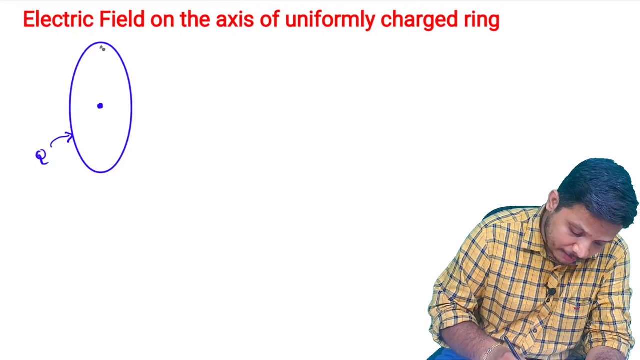 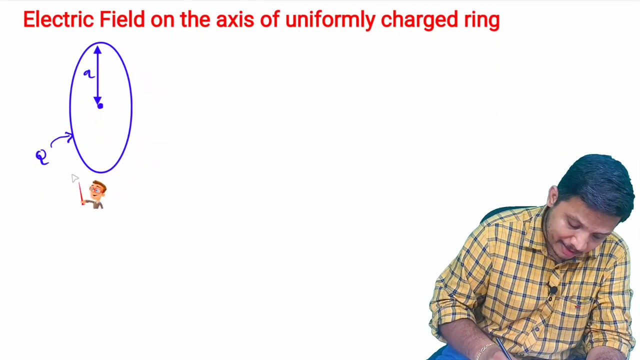 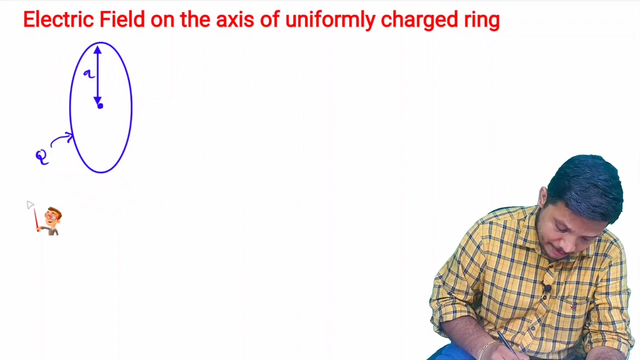 Welcome to Electromagnetics Theory lecture series. Hi, Professor Hitesh Dholakia is going to explain you. electric field on the axis of ring due to uniformly charged ring Right. So let us have one ring first. Now in this ring let us deposit charge Q on it Right. And this is what center of ring. Now let us say radius of this ring is small, a, Then line charge on this ring, that will be total charge divided by length, and length will be 2 pi a. 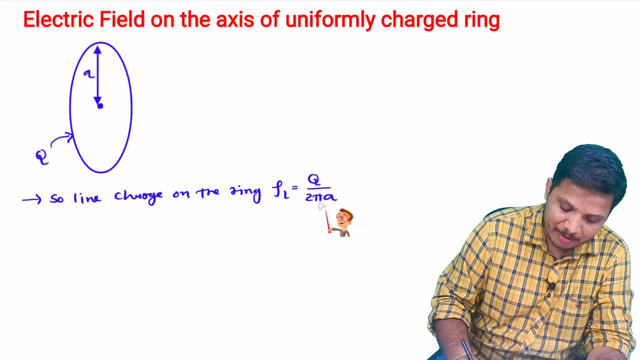 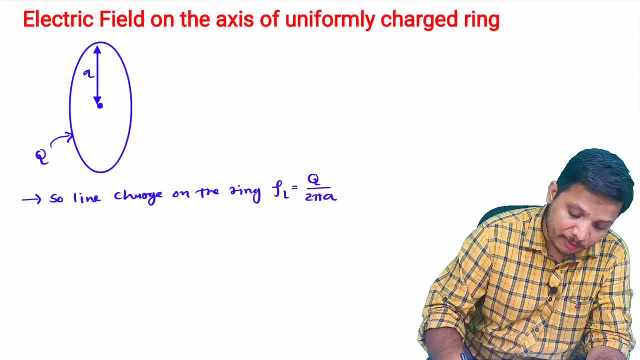 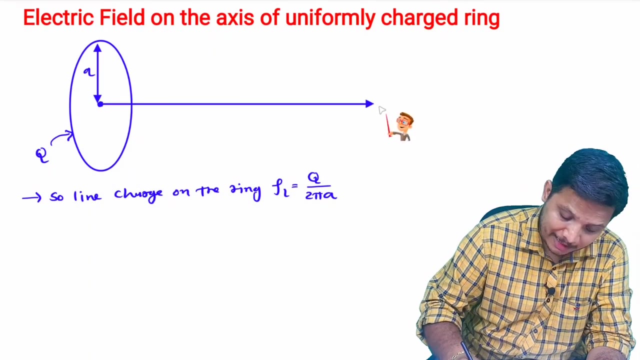 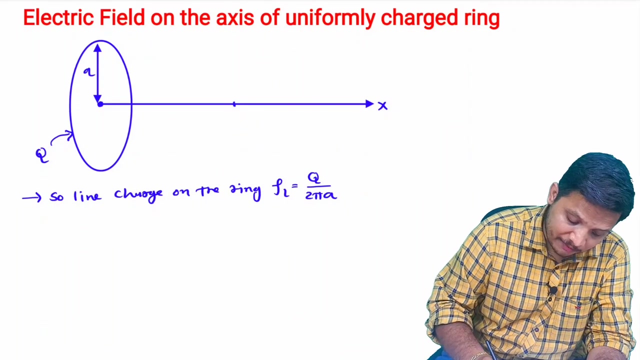 So line charge will be total charge Q divided by 2 pi a. Now our agenda is to identify electric field on the axis of uniformly charged ring. So axis of the ring, that is this. Let us say: this is what x axis which we have, And our agenda is to identify electric field somewhere over here, Right? So let us say: 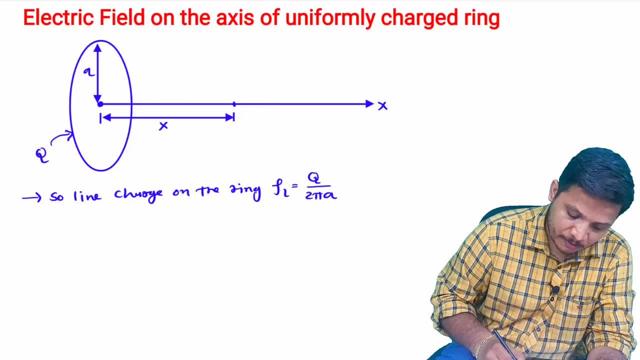 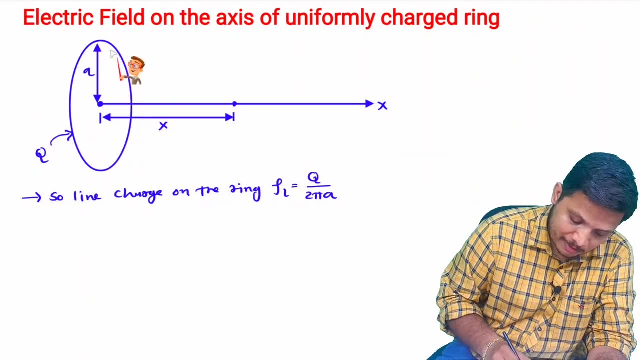 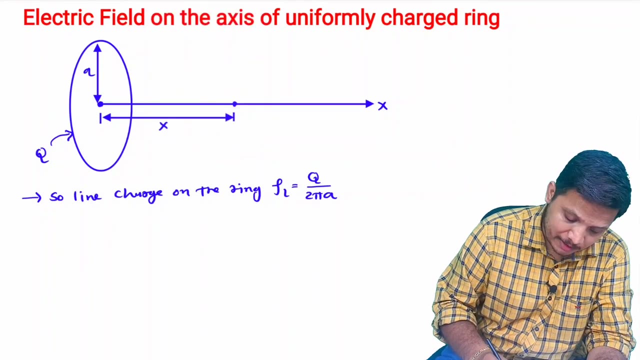 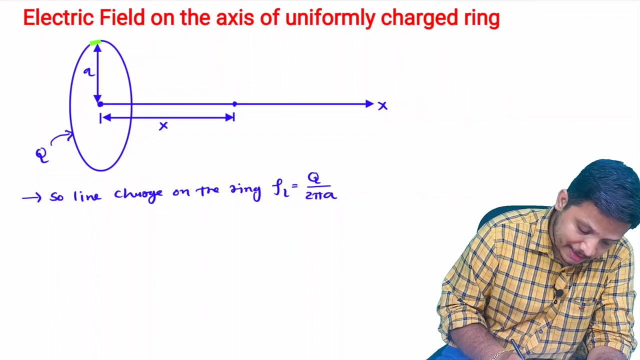 distance with respect to center is x. So at this location we are delivered to find electric field because of this uniformly charged ring. Now to have this derivation, let us consider first small differential element over here. So I'm considering small differential element. Let us say this is having charge dq, So this dq charge. 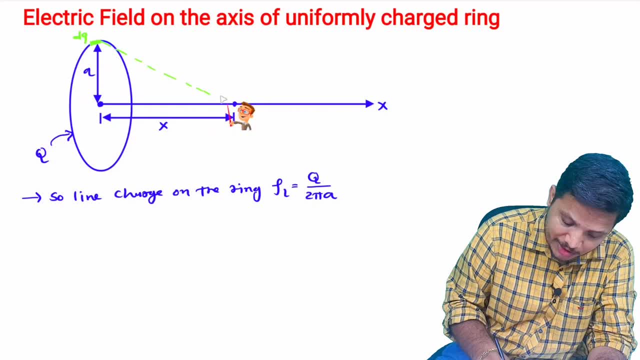 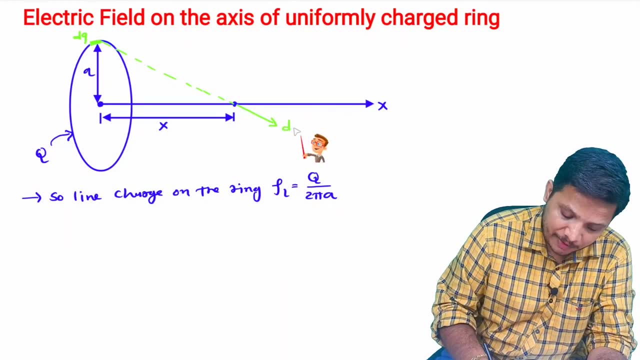 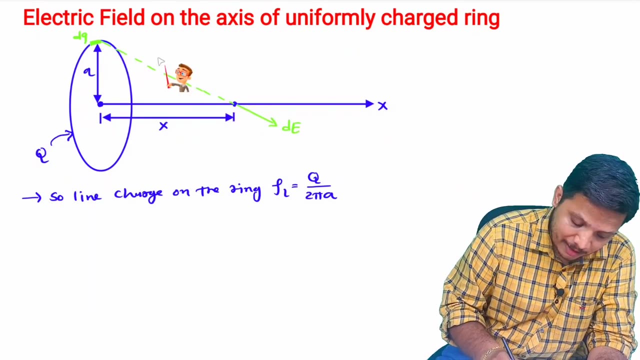 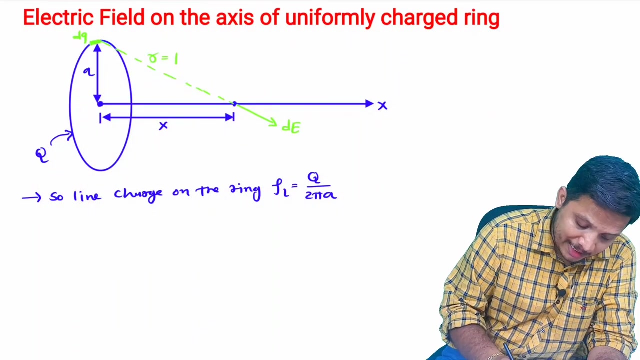 that will be resulting into electric field at this location, you see, in this direction, Right? So electric field. let us say that is dE, Then how much value is there with dE? So that is based on this distance, And this distance is how much? Let us say it is r, So that r will be as per this triangle. we can say: r is square root of x square plus a square, Right. 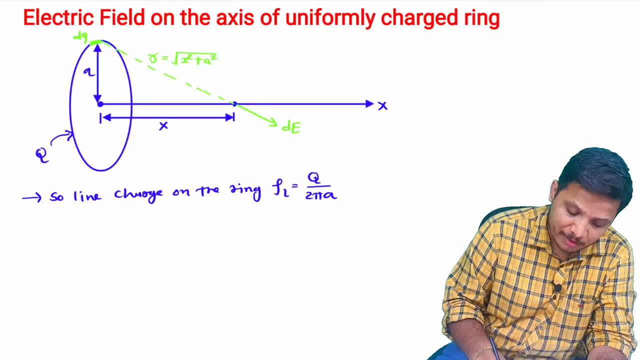 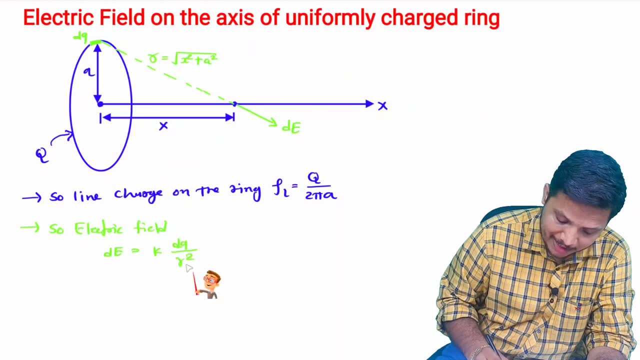 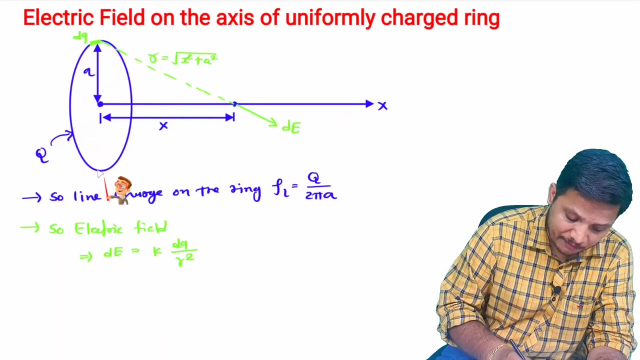 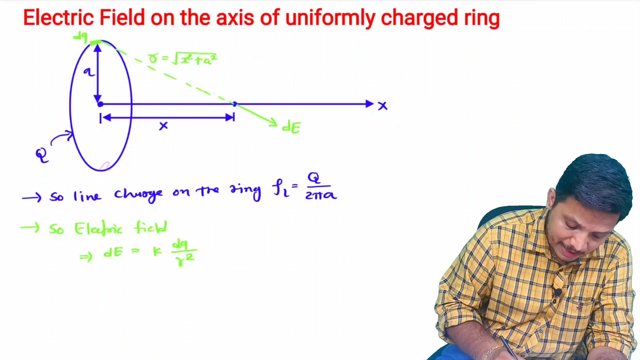 So electric field dE. at this position that will be k dq by r square Right Now. see, our agenda is to find electric field due to complete ring Right. So now one more assumption that one should know. See if I exactly opposite diametric point is being considered. 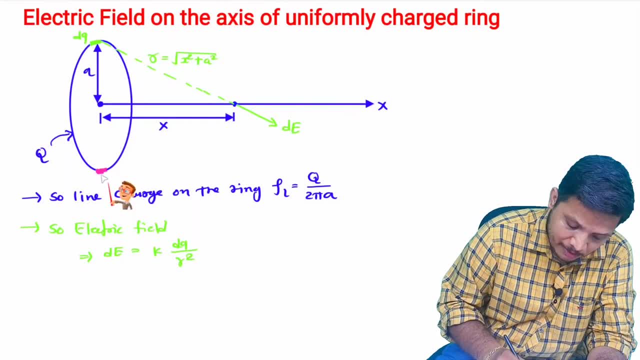 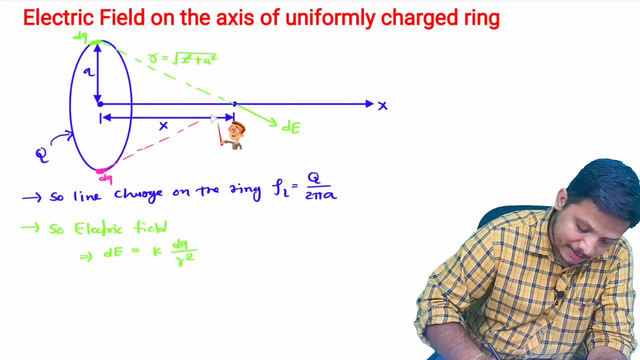 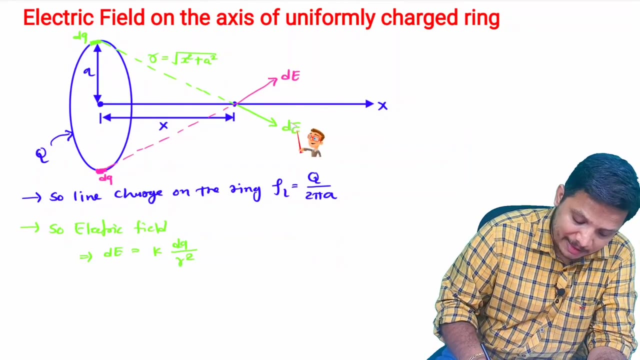 in that case, see this differential charge dq that will form electric field at this location, like this. you see, And if I say magnitude wise, then this dE and this dE, both are same. Now, if you say this angle is theta, then this angle, that has to be also theta. Now, if you say this angle is theta, then this angle, that has to be also theta. 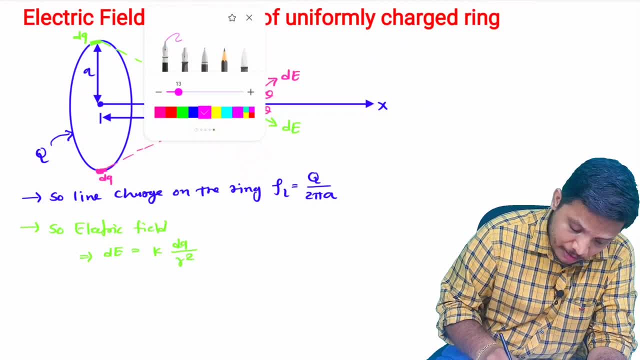 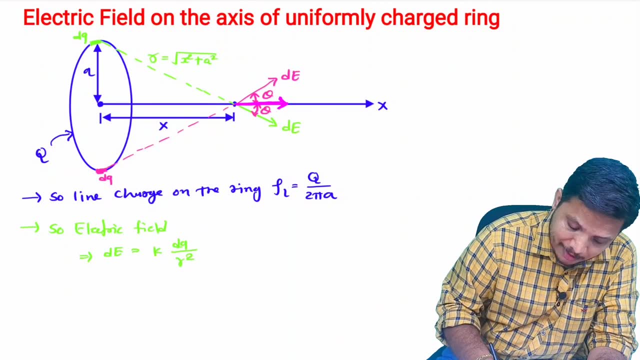 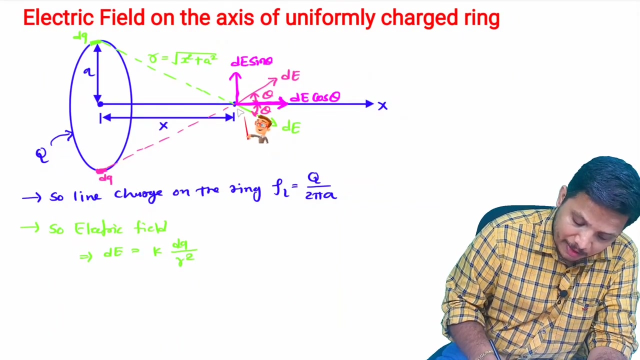 Now, if you analyze this with respect to components, then you see in this direction components are getting added And this component is dE cos theta. But if you see component wise, then in this direction component is dE sin theta because of this electric field and component wise, this will be dE sin theta. 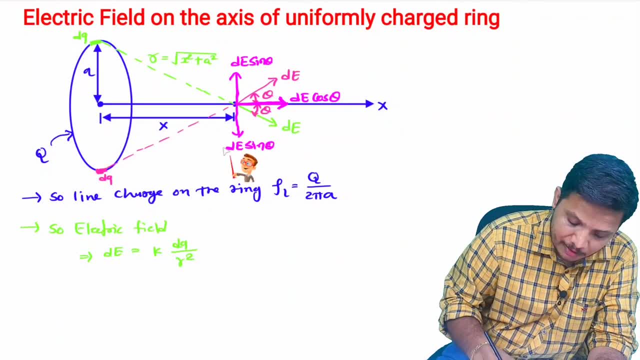 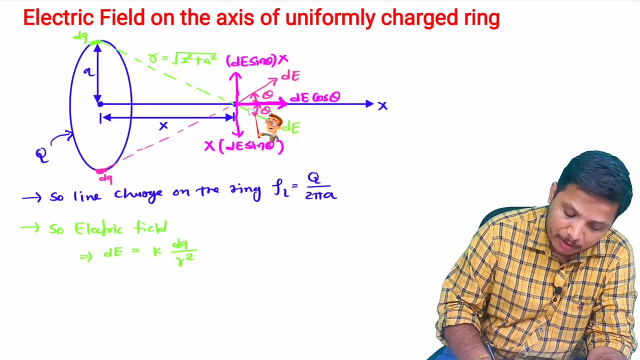 And if you see component wise, then in this direction. component is dE sin theta. But if you see component wise, then in this direction. component is dE sin theta. Without these, only dE cos theta that is available. So that will get canceled. So sine component is not present. So what we can say electric field is having only cos component. 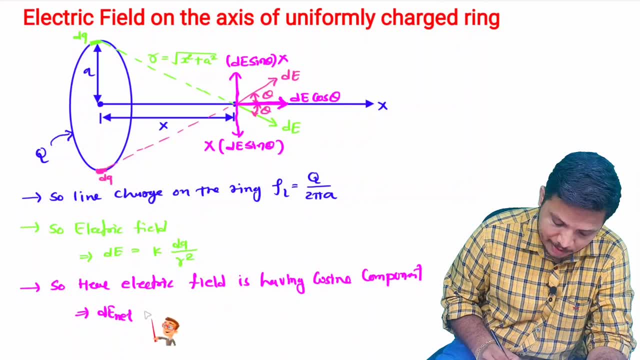 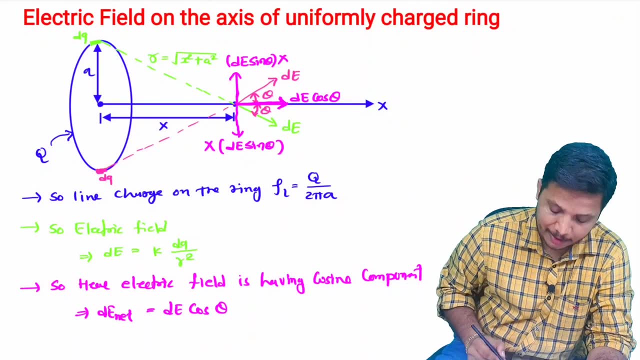 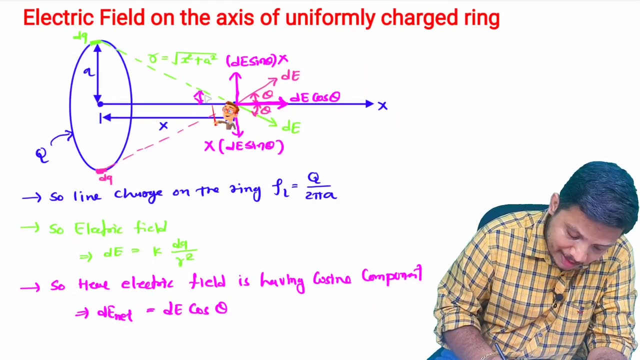 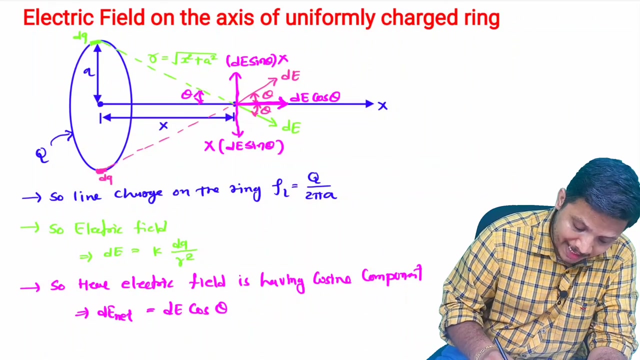 So I can say: net electric field due to small differential charge, dq, that is dE, cos theta. now let us calculate cos theta. so see, this angle is theta, so obviously this angle that has to be theta. now consider this triangle. so based on this triangle, all I can say is cos theta that is adjacent, that is X divided by. 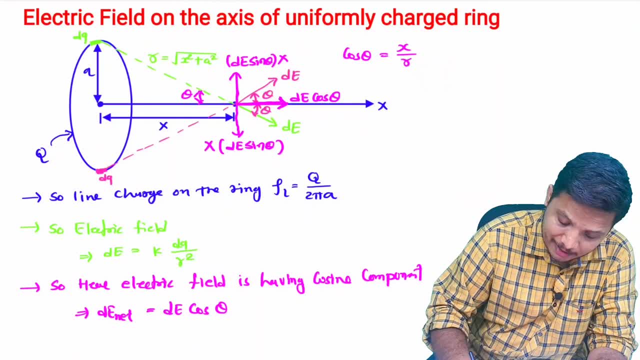 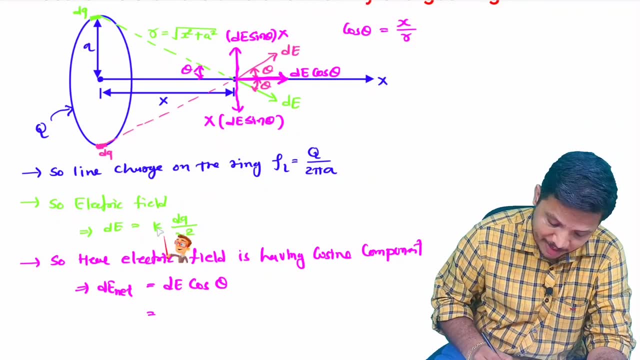 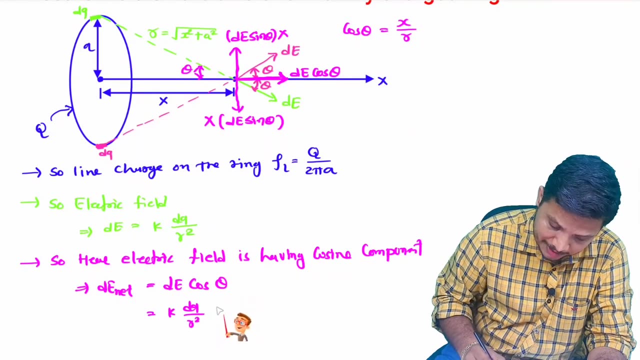 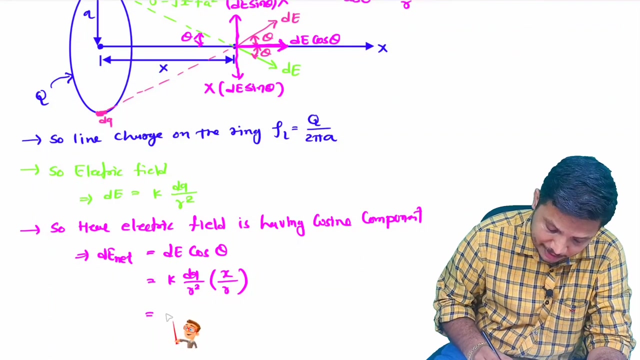 diagonal, so X by R. that I can say right. so now if I substitute cos theta over here, then we'll be having DE, that is this K d cube by R, square into cos theta, that is X by R. so I can say this net electric field, that is K X d cube by R. 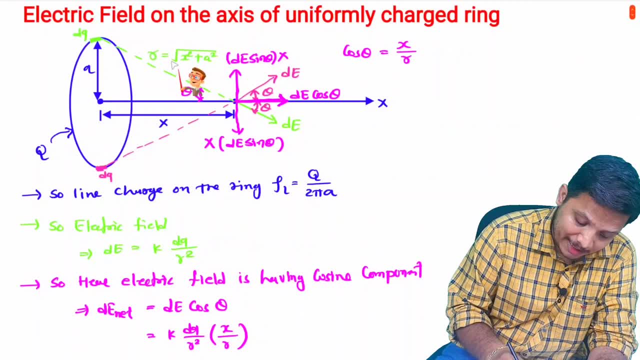 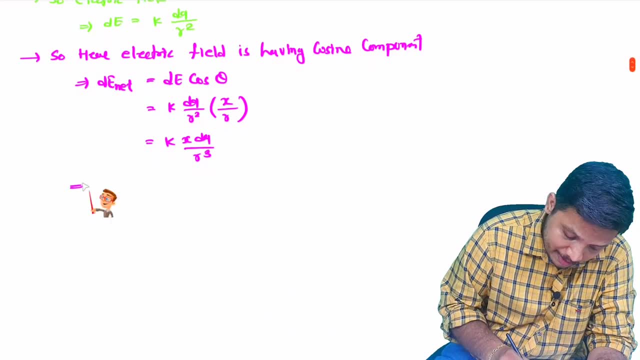 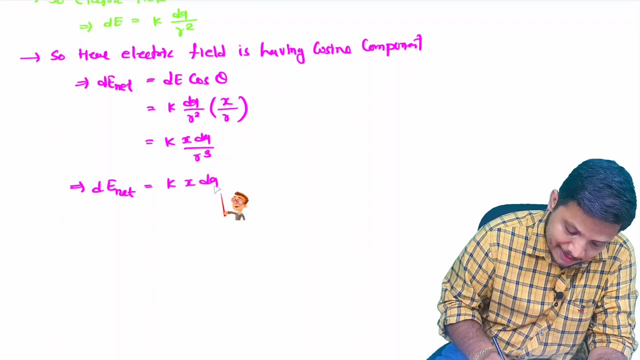 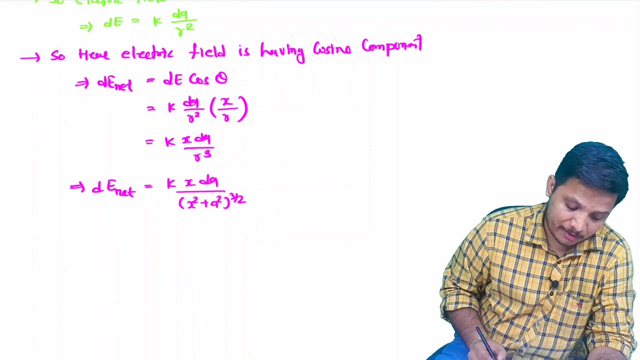 cube where R is how much, where R is square root of X square plus Y square. so if I place these values I'll be having small differential net electric field, that is K, X, d cube divided by X square plus a square raised to 3 by 2 right. and if you 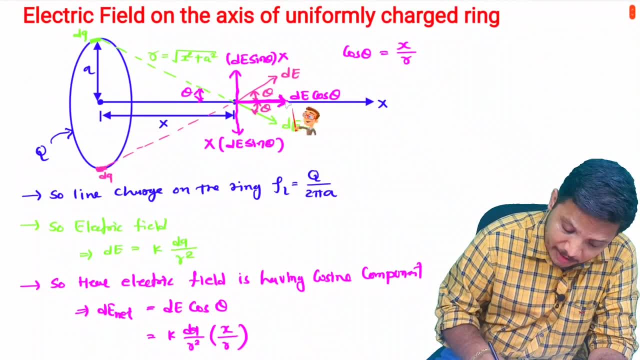 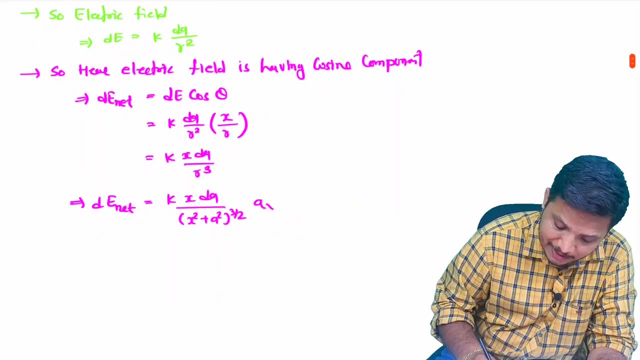 observe direction, then direction of this electric field will be the direction of this electric field will be the direction of this electric field that is there in the direction of axis right, so that is there in the direction of axis. here direction of axis is AX. so I'm writing by. 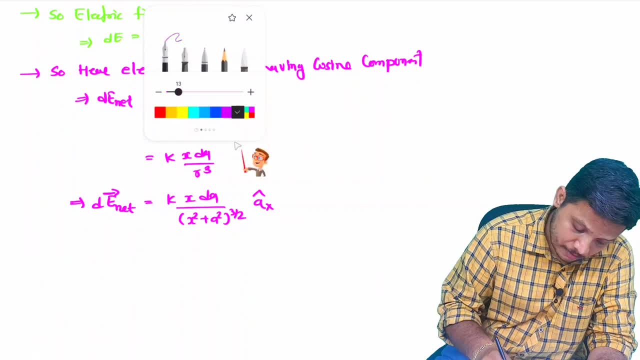 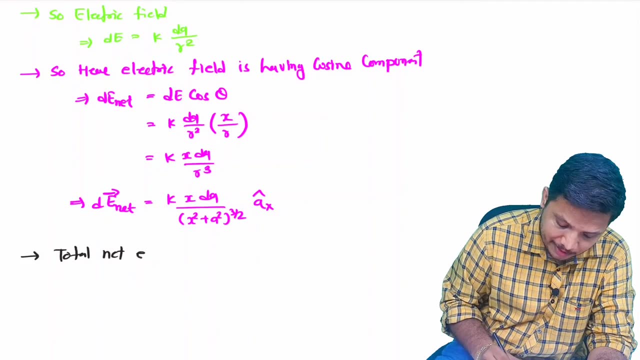 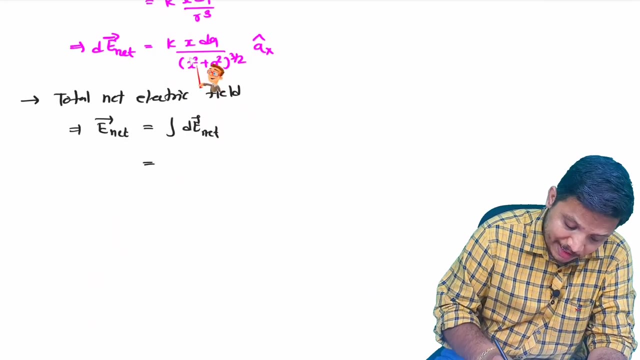 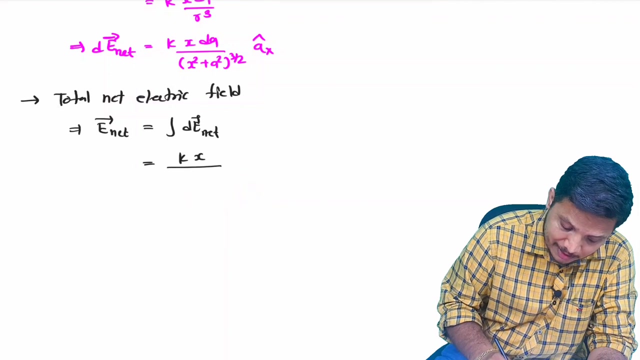 direction. it is there in AX direction. now, if we want to calculate total electric field, so total net electric field, so that will be integration of this. so if you do integration, then what will happen? so if you do integration, then what will happen in that case, you will be observing this- will be K, X divided by X square plus a. 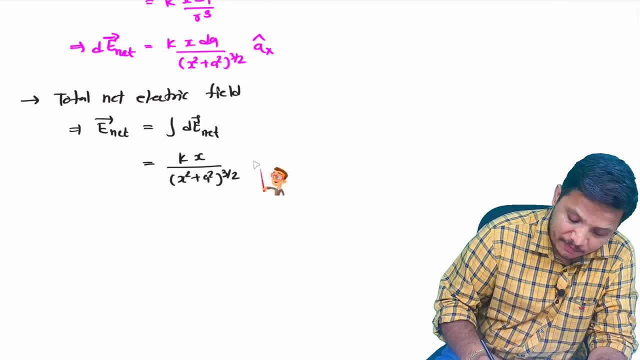 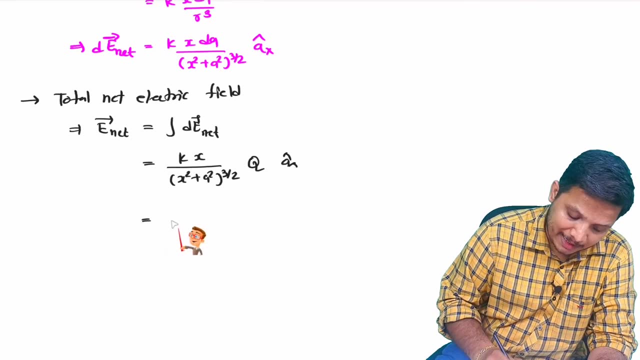 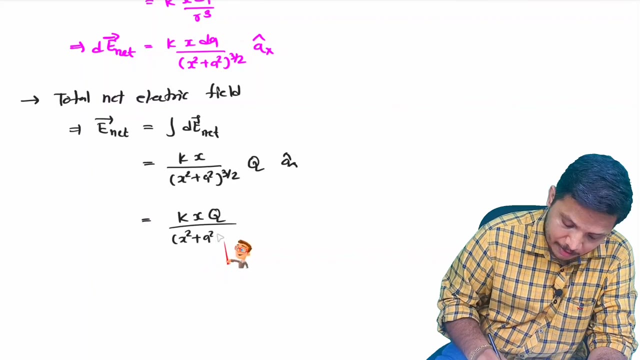 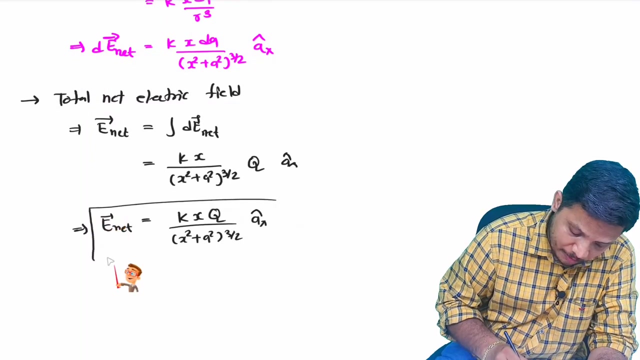 square raised to 3 by 2 and integration of D Q, that will be total charge Q. so I can say this net electric field that is K X Q divided by X square, plus a square raised to 3 by 2 in AX direction. now this is the basic formula that one should remember right and sometimes there. 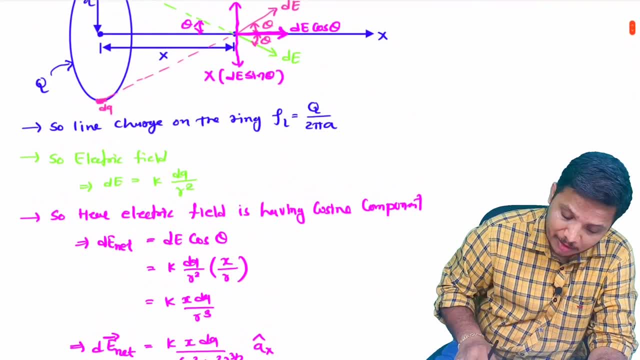 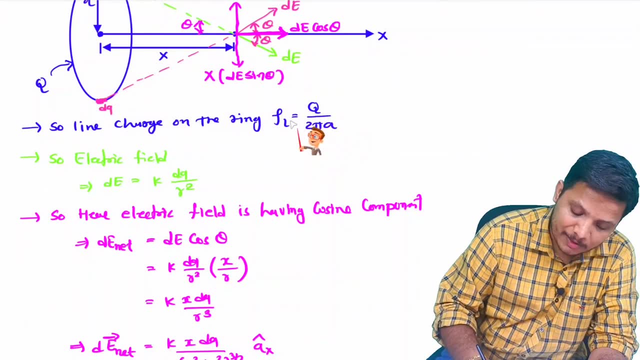 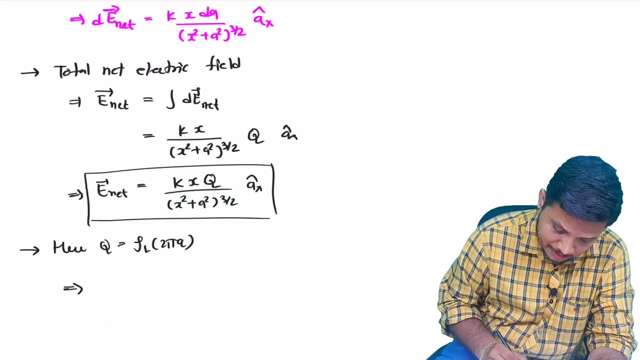 can be one more formula, which is there, based on line charge density, right. so, as we know, line charge density, that is Q by 2 by 8. so Q is equals to Rho L into 2 by 8, and if you place this then you will be having net electric field. that will be.